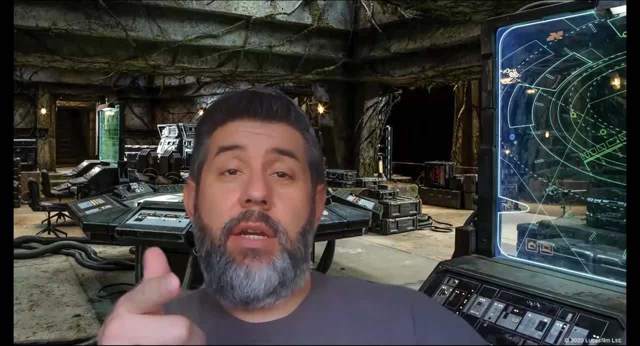 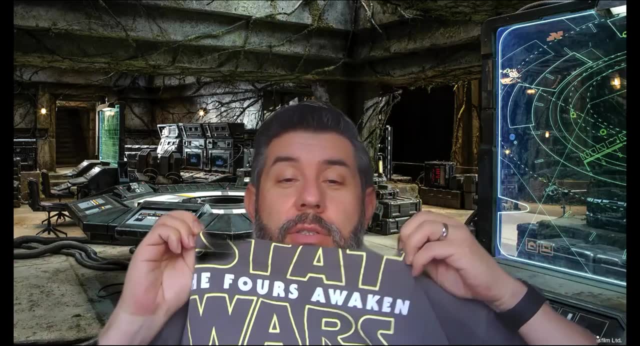 Hey guys, Mr Maez is here. How you doing out there. You see I got my Star Wars background. It's May 4th. May the 4th, be with you. Got my Star Wars. It says Stat Wars. It's not really a. 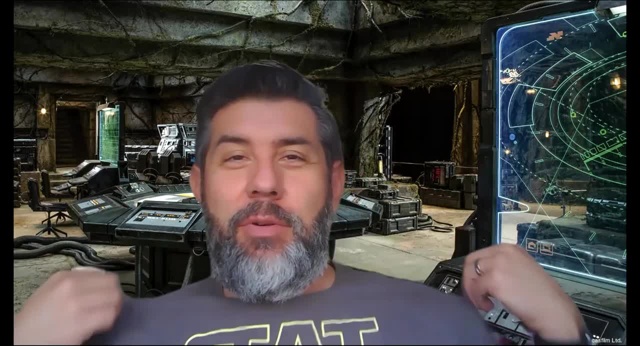 Star Wars t-shirt but it says it's like Star Wars, It's a play on Star Wars, Stat Wars. Anyway, we're doing stats today. Welcome, We are looking at So on this video, what I wanted to do is I. 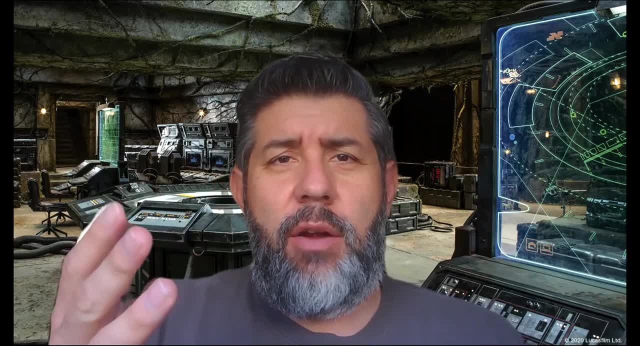 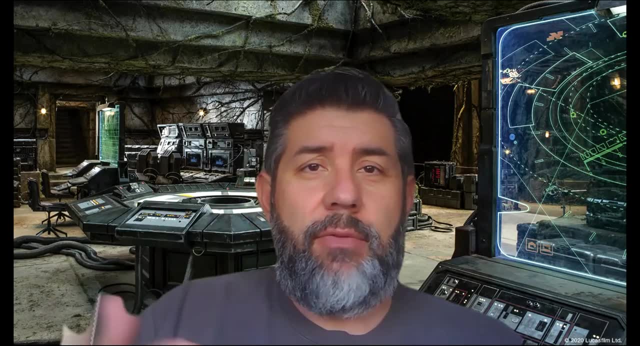 wanted to go over something that kind of confuses some students here and there quite often, And that is: how do we make a conclusion on a hypothesis test on inference? So how do we make an inference on the population based on a confidence interval? And a lot of times I'll ask this question in my 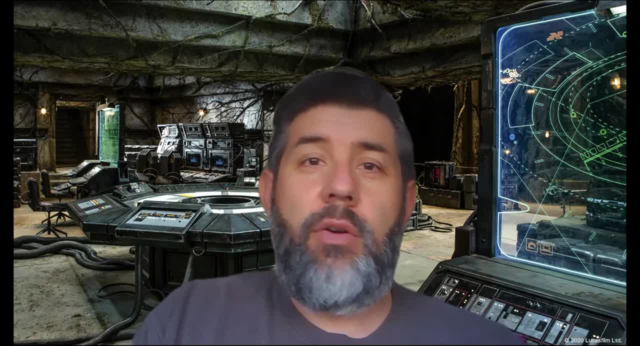 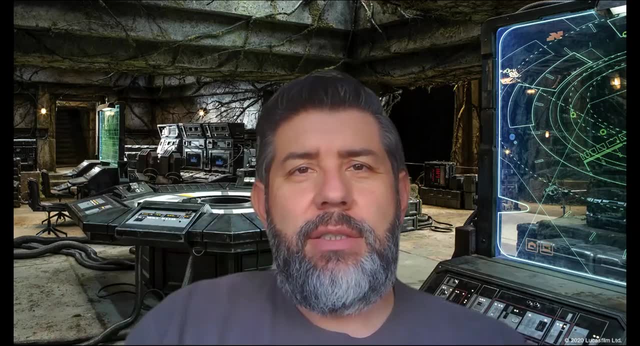 stats classes. What does this confidence interval tell you about this? Does it give you evidence of this situation occurring? So we're not doing a complete hypothesis test in this case. We're just looking at the confidence interval and seeing if we can tell something about whether we would fail. 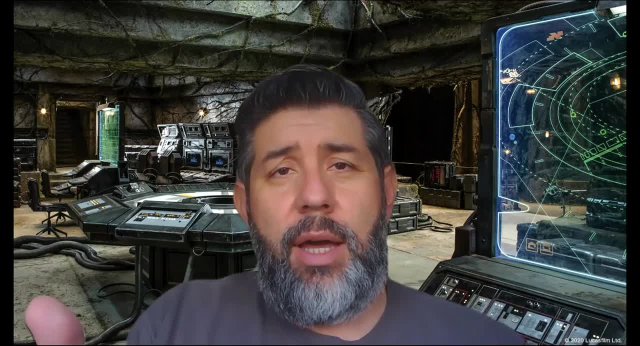 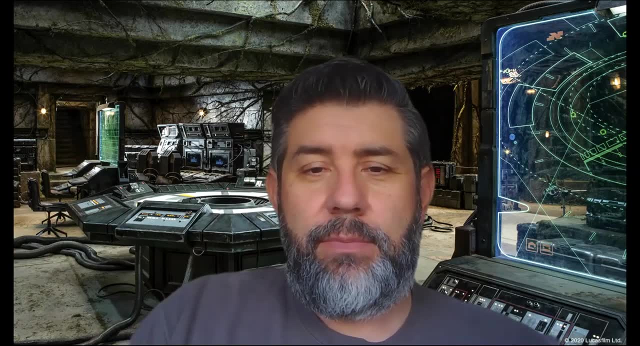 to reject or reject a null hypothesis? Have we been doing a hypothesis test the whole time? So let's take a look at that and I'll kind of run through this idea very quickly, All right, So here I have an example, and you know I should. 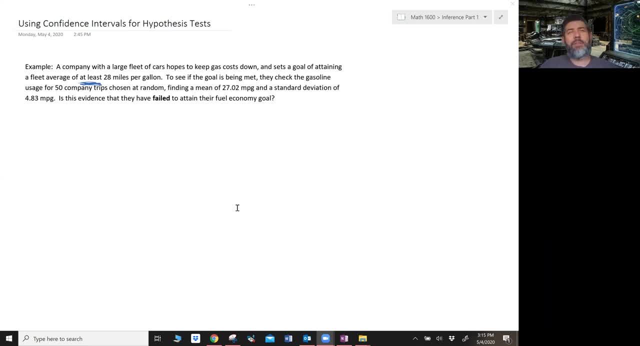 have said like a Starfleet, right? No, that would be Star Trek, like a rebel fleet or something like that. But we'll just talk about cars here And what we want to do is we want to have a goal, having a fuel efficiency goal of at least 28 miles per gallon. So we're going to have at least 28 miles. 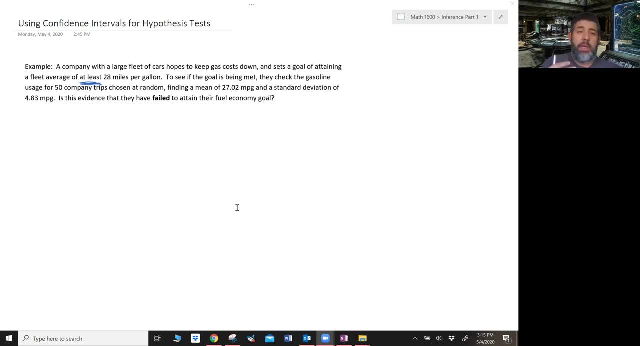 per gallon. In order to meet this goal, the company does a sample size of 50. They randomly select it. They find a mean of 27.02 miles per gallon and a standard deviation of 4.83.. Is there evidence So? 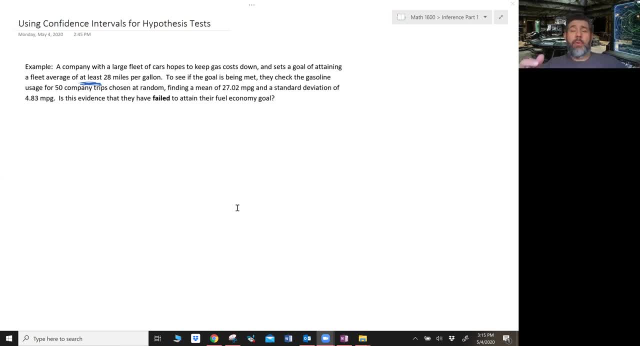 anytime we see evidence. you've seen my other videos where we're talking about confidence, sorry, hypothesis testing. Anytime it says: is there evidence. we're doing a hypothesis test, some sort of inference procedure. The question here is: is there evidence that they've failed to attend their economy goal? So let's first talk about 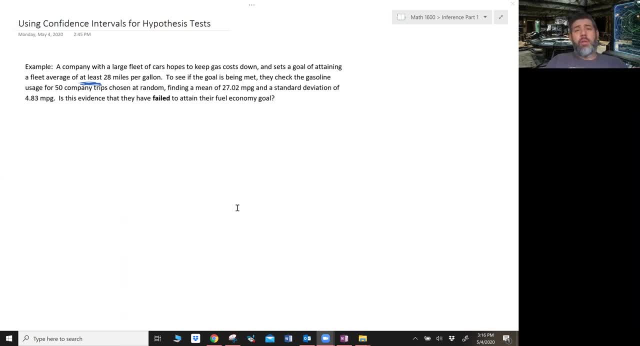 the hypothesis test. So if we were going to write a null and alternative hypothesis, what would those be? Well, our null hypothesis- let's see if I'm writing here. Our null hypothesis is going to be: mu is equal to 28 miles per gallon. 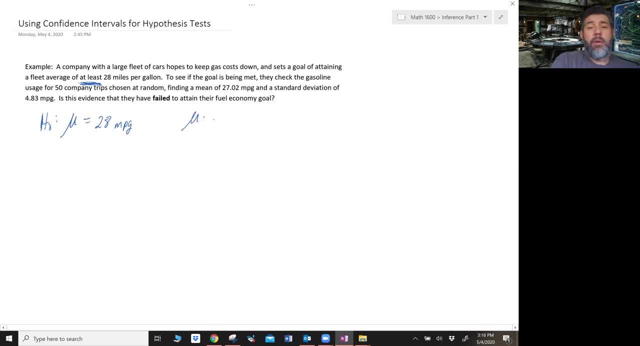 That is a kind of our null hypothesis. So if we were going to write a null and alternative hypothesis, our baseline right Mu here is going to be our mean miles per gallon for all cars in the company. And I know if my handwriting is bad, sorry about that. 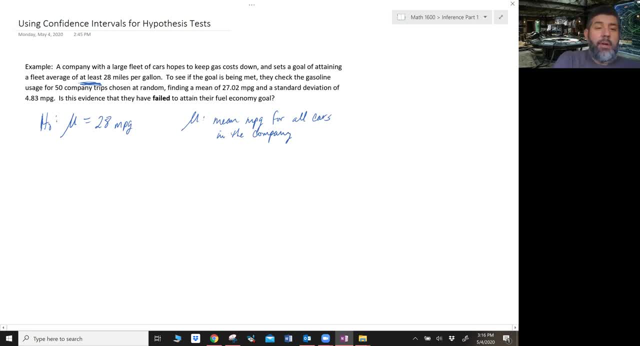 You know, and our alternative hypothesis is going to be, mu is now, they need to have at least 28 miles per gallon. So if they have failed to attain their goal, that means that 28,. if they do not meet their goal of 28 gallons, so that's going to be less. 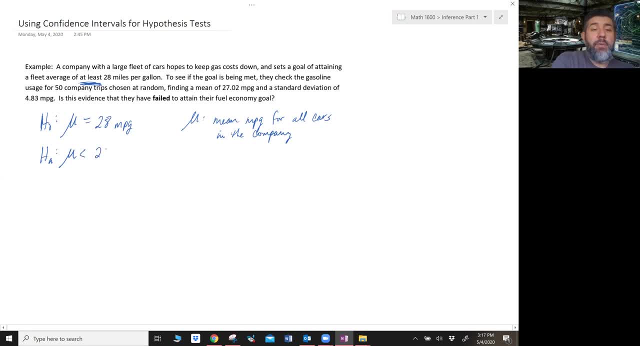 than 28.. So I'm going to say: mu is less than 28 miles per gallon, So this would be evidence that they did not meet their requirement. Okay, So they failed to meet it. So that's why we have that bold fail, All right. So now, if we were going to do a hypothesis test, what we would do is we would: 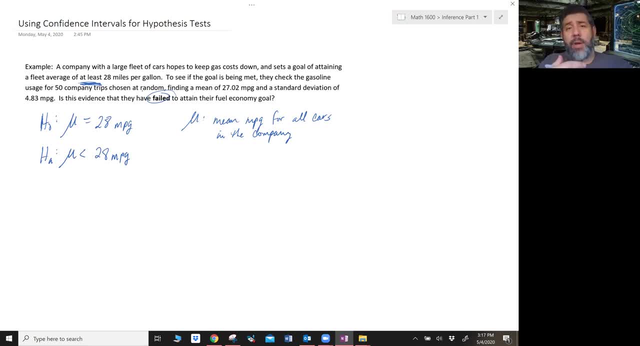 next, do our conditions for inference, which, by the way, you have to write those conditions, whether you're doing a hypothesis test or the confidence interval, anytime you have inference procedures you have to do the confidence, the conditions. So, really quickly, just the conditions. random, a random sample. 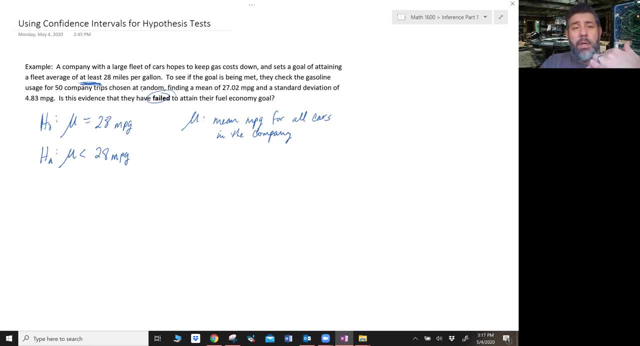 So we did. we chose a random sample of 50 company trips. We have to have independence. We'll assume that each trip is independent of one another, And we can also assume that 50 trips is less than 10% of all trips that we've taken in that company. And then, finally, we want to have our 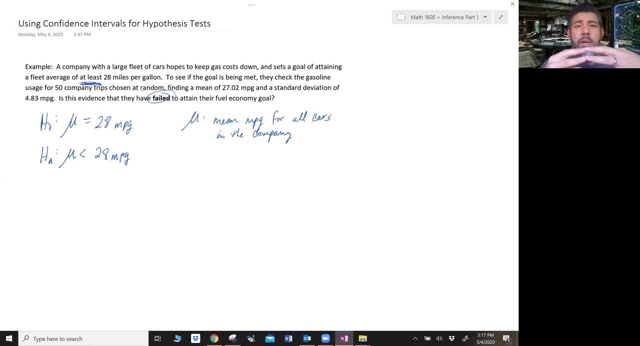 sample size greater than 30. So that's the central limit theorem here down. So since, since our N, our sample size is greater than 30, we can apply this very easily to our, to our problem here. So that would be one way that we can fill that. condition is that our sample size is greater. 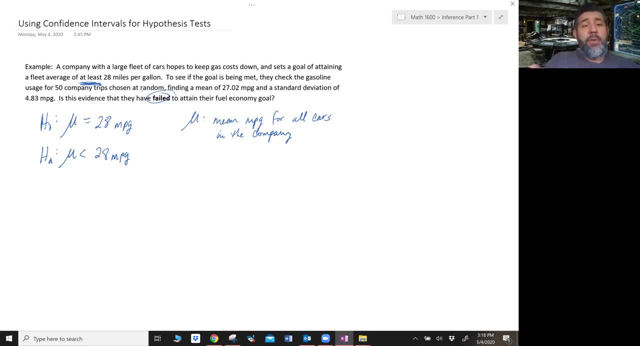 than 50. So since we have our conditions going satisfied- and I don't write them down, I just want to kind of move on. Now here's what I want to do. I would like, since this video is really about using a confidence interval, to talk about this hypothesis test. let me create. 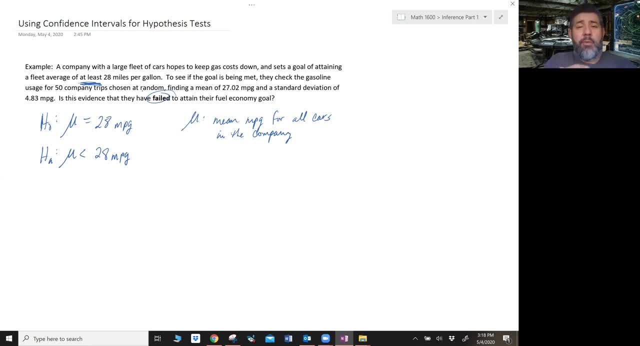 create a confidence interval. Now, this is a one sample T interval, because I have only one sample right. I have um N is going to be 50, and I have um X bar which is 27.02.. And I have 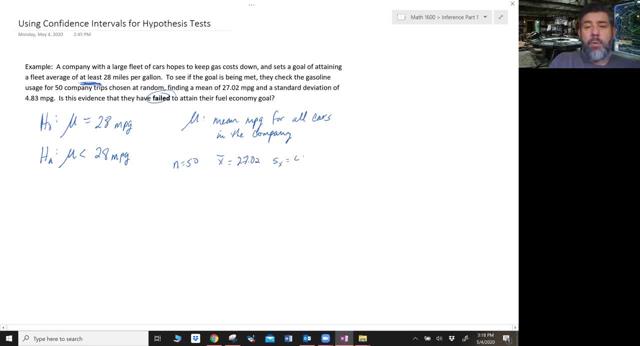 the standard deviation of 4.83.. And so what I'm going to do is I'm going to make a confidence interval. Now, um, let's suppose that my alpha level here is 0.05.. So if if I'm going to do a five percent alpha level, I'm going to need to know what confidence interval I 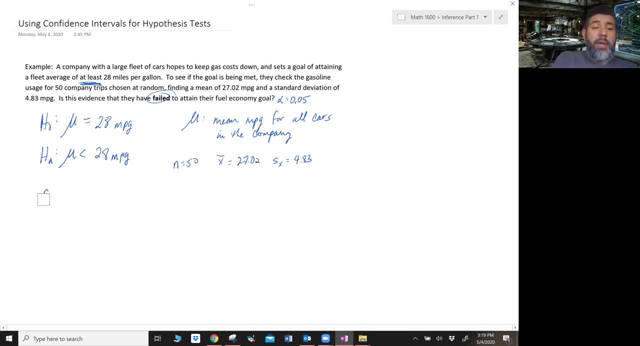 want to choose based on my alpha level And the way this works, is that? um, just very, very quickly, Let's see if I can draw. if this shows, hopefully this shows up here. Um, if I'm looking at the, 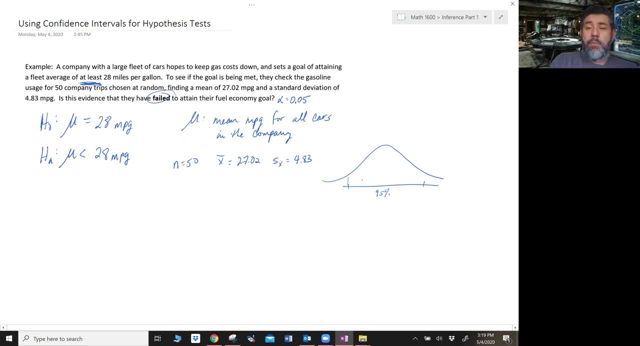 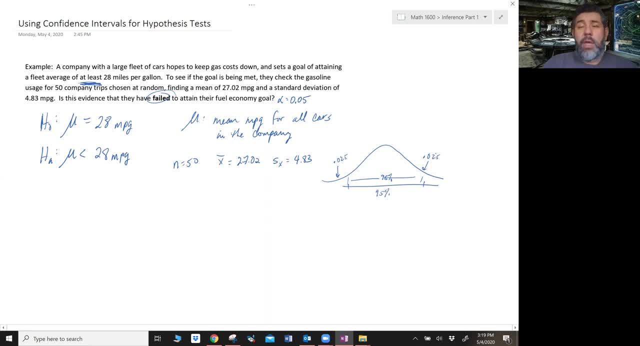 Here and 0.025 here. Then I have to look at the type of test. Am I running a one-tailed or a two-tailed test? A one-tailed test would happen if you one-tailed test would happen if you have a greater. 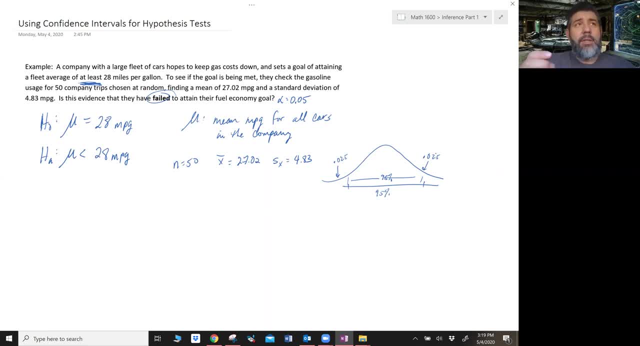 than or a less than in your alternative hypothesis, And a two-tailed test would be if you had a not equal to sign. So since I have a less than sign here in my null hypothesis, in my alternative hypothesis I'm talking about this area here, which is a lower tail, So it's a one-tail lower. 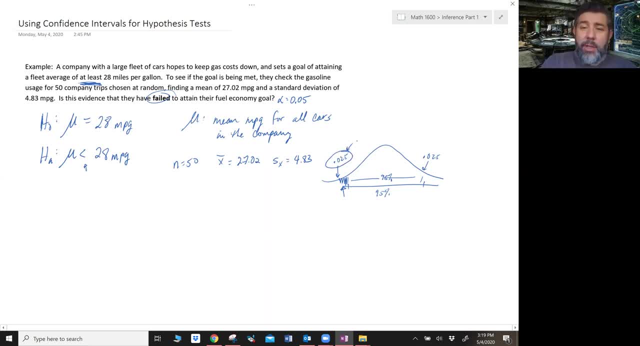 tail test. This is my alpha level. All right, So that's how I can tell my alpha level of a confidence interval. I can tell my confidence level or my alpha level. Sorry about this. So this would be my alpha level, that corresponds to a 95% confidence interval. Now I don't know. 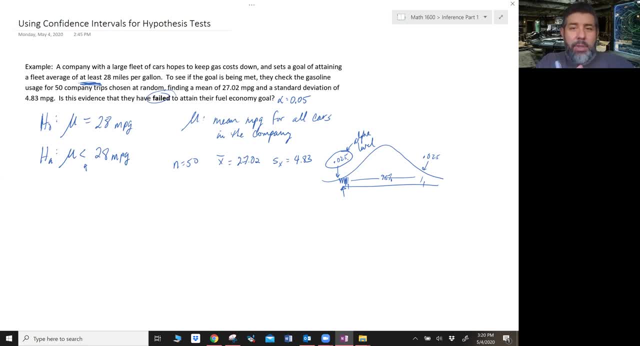 what confidence level I want in this. So I kind of have to work a little bit backwards here. So I do know that I have a 95% alpha level. So, using the same idea, using the same idea I have, let me just draw this. 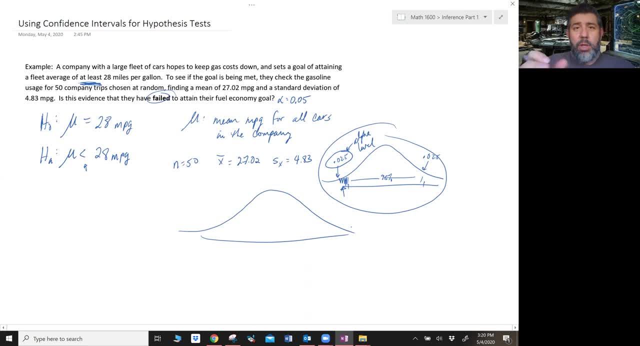 normal distribution and a normal or a T it's, it's. we're going to have a degrees of freedom here. In this case, our degrees of freedom, since we're using a T test, a T interval, is going to be 49, but I'm I don't know what percent here that I want in my confidence interval. How, however, 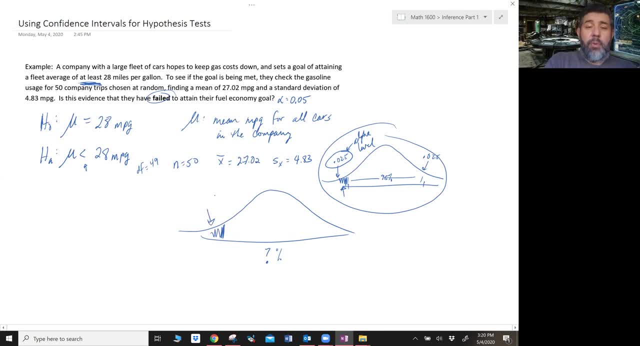 I do know that this alpha level is 0.. 0.05, based on the fact that I have a one tail test. Well, this is 0.05.. Then the upper tail has to also be 0.05.. What's left over in the middle of 0.05? 0.05 is 0.1. 0.1 minus one minus 0.1 is. 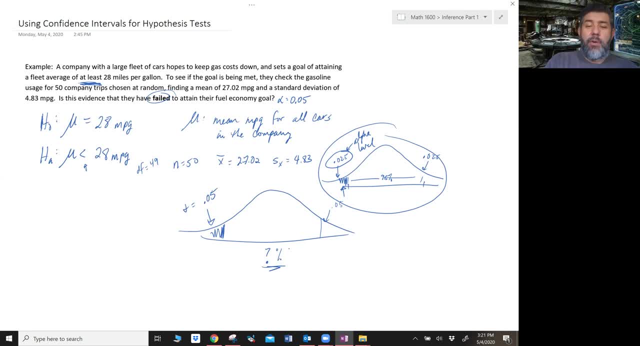 that's right, 90%, So I can get that. I need to create a 90% confidence interval So I can do this both ways. If I know the alpha level I can create. I can know what confidence level I'm going to use to create If I know the confidence interval and the confidence level. 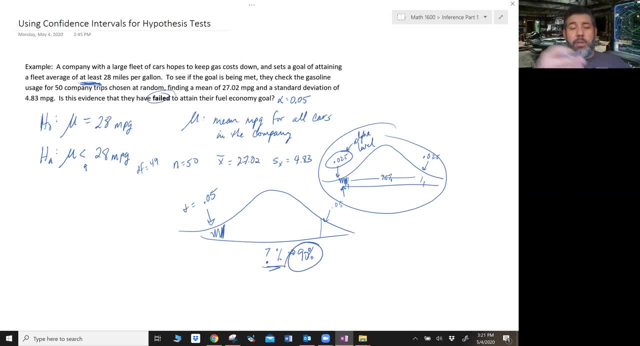 I know what alpha level that I'm going to need to test this on. So right now we're just going, we're going to use a 90% confidence, based on the alpha level that I have, and I'm going to create a 90% confidence interval. So just reminding you what that is, 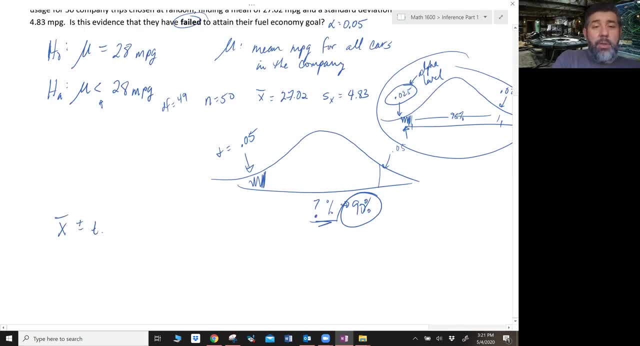 X bar plus or minus T star. We're using 49 degrees of freedom times S over root N. Okay, So we've got 27.02 plus or minus, and I'll get that in just a second S, which was 4.83 over the square root of 50.. 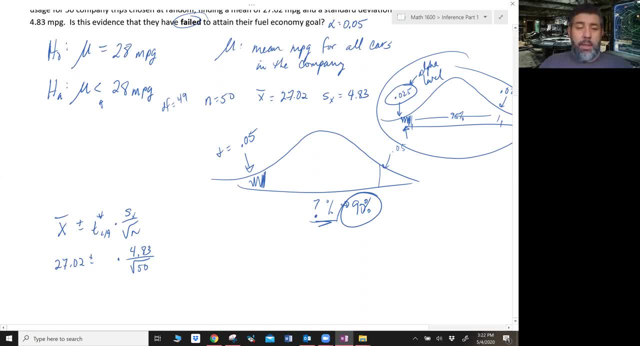 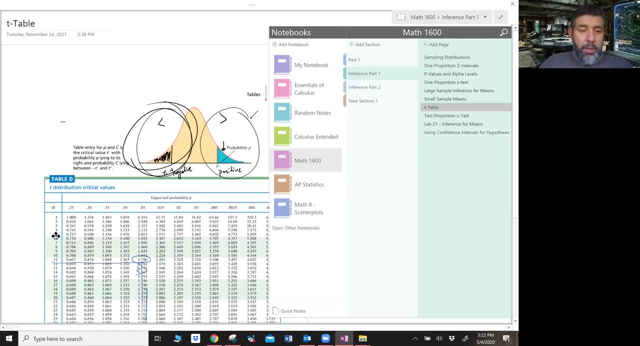 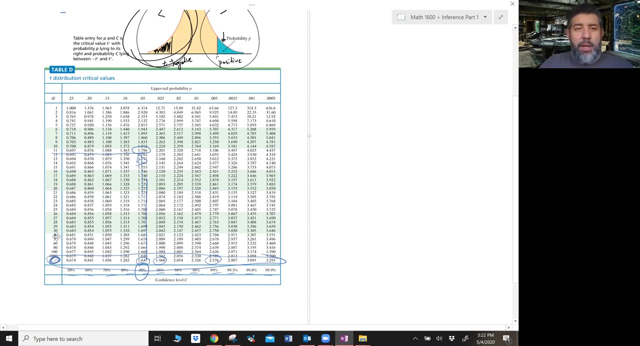 Okay, So we want to get 49 degrees of freedom. So I'm going to quickly go to my T table here and I have 49 degrees of freedom, which is close to 50. You know, once we get over 30, the D, it's kind of hard to find that, that critical T value. 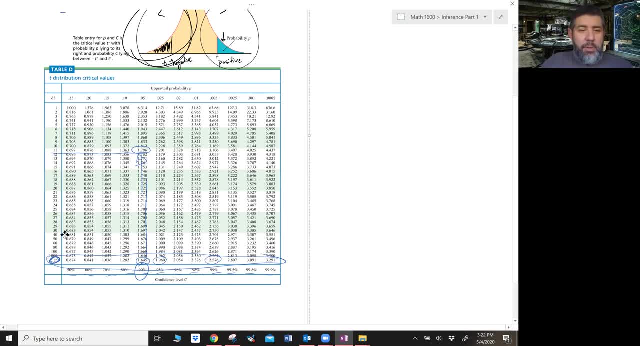 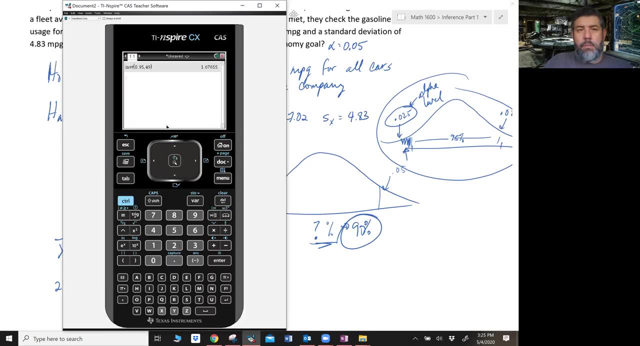 In fact, I probably want to use a calculator to do that. In fact, I will use a calculator. So give me a second and I'm going to use a calculator. So I have my calculator here and I did an inverse T. So I did an inverse T distribution. I have 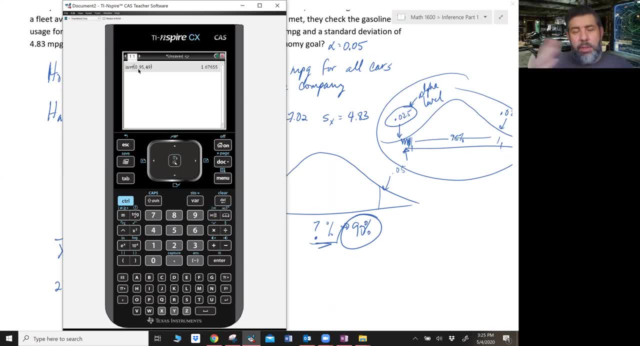 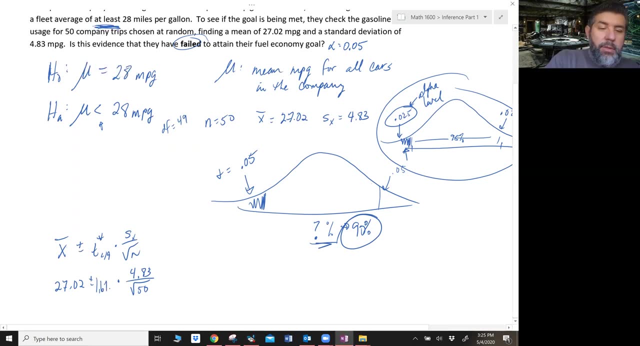 95%, because I have a 5% alpha level which, subtracted as one is 95 with 49 degrees of freedom, is going to give me 1.67655.. All right, So I'm got 1.6, 1.67.. All right. And you know what, since I have the calculator here, 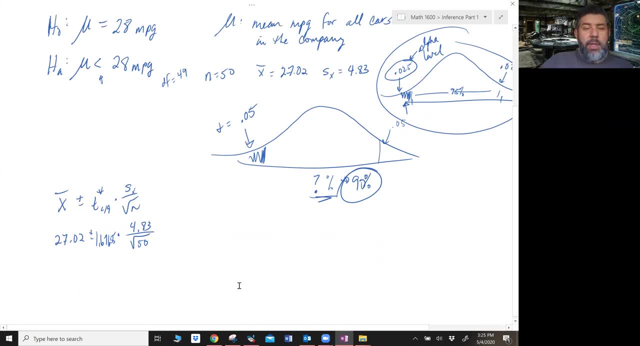 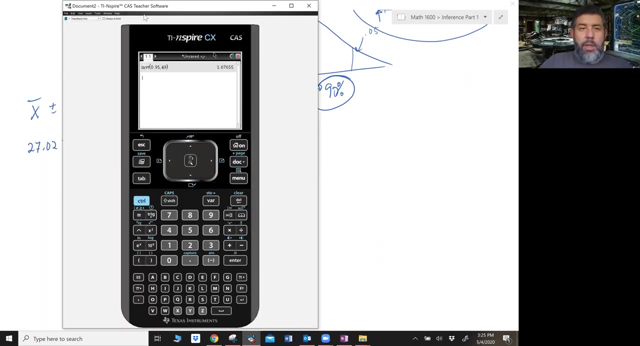 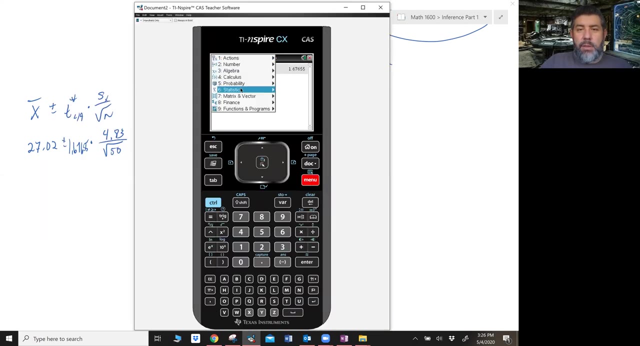 I'm going to just use the calculator to to um, to calculate this, to go and count my, I don't know why my calculator shrinks so much. All right, So we're going to do a one. statistics: confidence intervals- T interval. 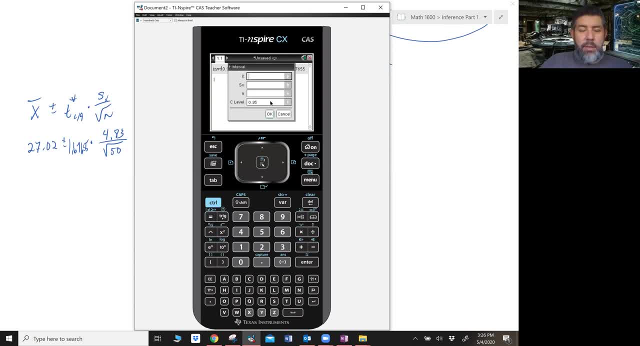 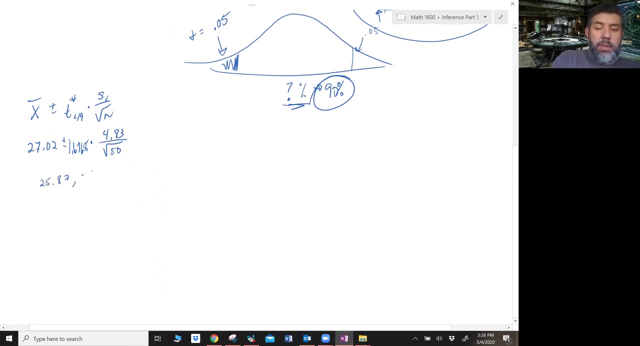 and we're going to use stats to do that. My X bar is 27.02.. My standard deviation is 4.83.. My N is 50 and we're going to go a 90% confidence level And we're going to have 25.87 and 28.17,, 25.87 and 20.. What was that again? 21,, 28.17.. Okay, 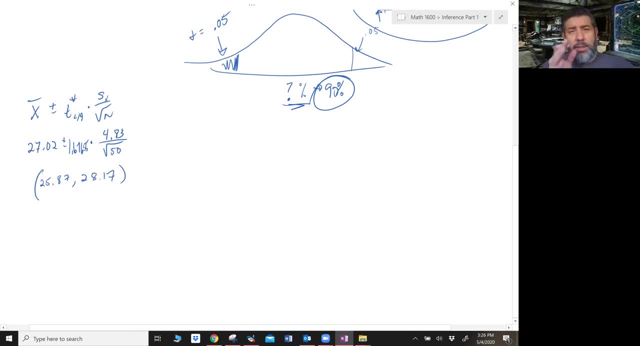 All right. So there's my interval. So so check this out. Check this out, guys. This is check this out, guys. We can't even talk today here. Uh, so check this out. What we're going to do is we're going to say: right. 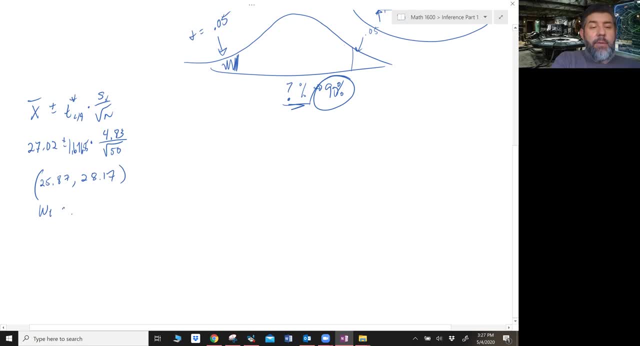 we always write this in context. We are 90% confident that the true mean- uh, what are we talking about? Miles per gallon is between: the true mean miles per gallon for all cars- All right, So all the company cars. the total amount of miles per gallon for all cars is between 25.87 and 28.1, seven miles per gallon. 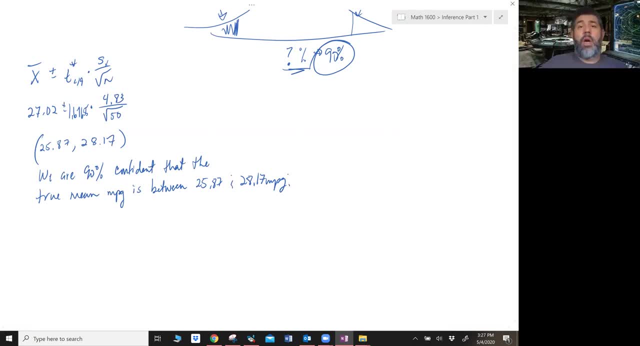 Now I'm going to- I'm just kind of doing this really, really quickly because I want to get to the point of this video. So the point of the video where we're a couple of things. the goal was one I didn't want you to see- where the PR, where the confidence level comes. 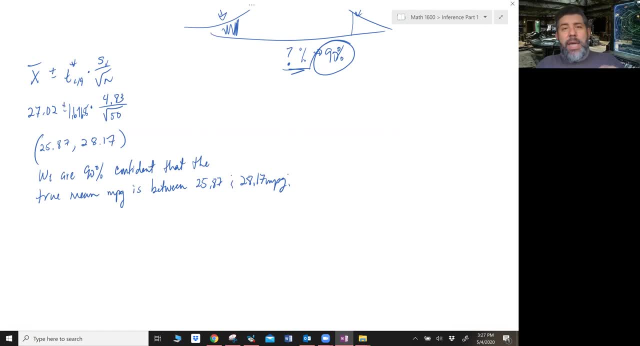 from if we're looking at an alpha level, and where the alpha level comes from If we're looking at a confidence level. The second thing is: how can we take our confidence interval And make an inference on the population or make a make an? 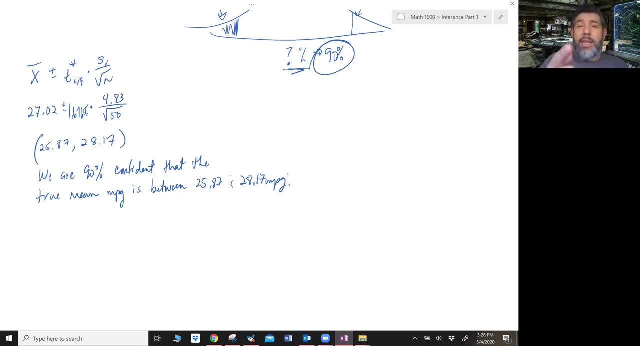 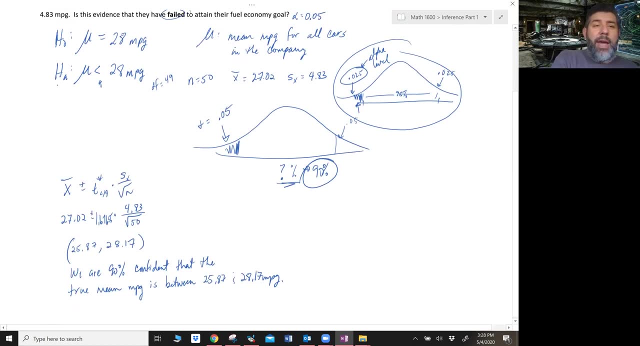 a conclusion of the hypothesis test based on our confidence interval. let's take a look at that now. so we've got. i'm going to shrink this down just a bit. here we've. we were trying to um have a. we were trying to have a null hypothesis that the mu, the mean, was less than 28 miles per gallon. 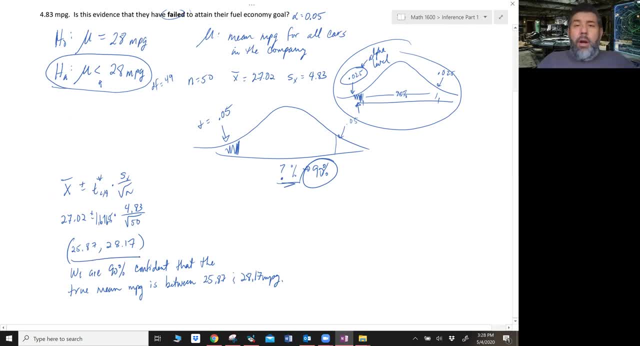 so we're going to look at is. we're going to look at our confidence interval and we're going to say to ourselves self: is the null hypothesized value within our confidence interval? the null hypothesized value is 28. is that within my confidence interval? yes, it is right, it goes. 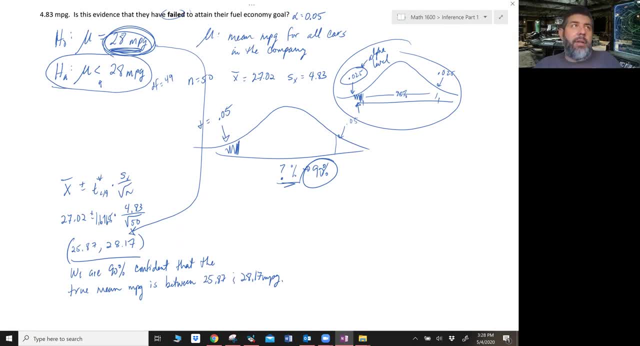 from 25.87 to 28.17. yes, i know it's only 0.17 and it's like. it's like more. there's more space in towards the 25 than it is towards the 20, but the fact that the 28 is within our interval tells us this. it tells us that, hey. 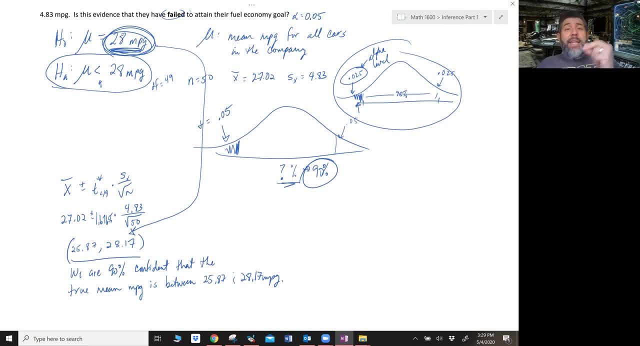 it is possible that 28 is our true mean. so if it's possible that 28 somewhere in there, possible that it doesn't tell the confidence, doesn't tell us like what the probability of being 20, it just tells us that it's possible, it is. if it's possible that 28 is in fact the true, 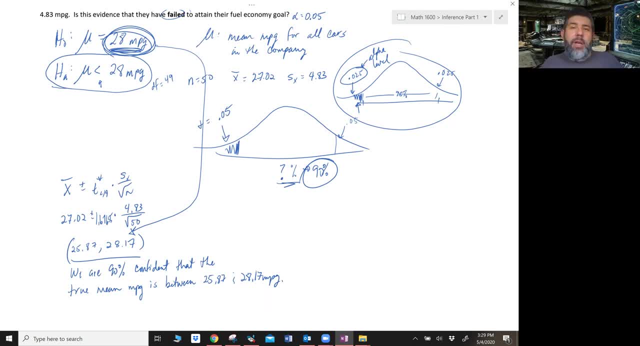 mean. so we're going to try to reject the null, because, look, the null is that it's equal to 28, so it could be 28. in fact, it could be 28.17, which, in that that case, is greater than 28, which is what. 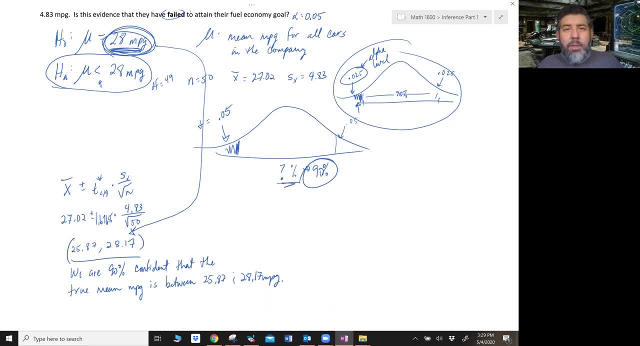 we wanted our. we wanted to be all less than 28 in our, in our um alternative hypothesis. so what i would do, based on this hypothesis, this confidence interval, is: i would say that, based on this confidence interval, i would fail to reject the null and i do not have enough evidence. 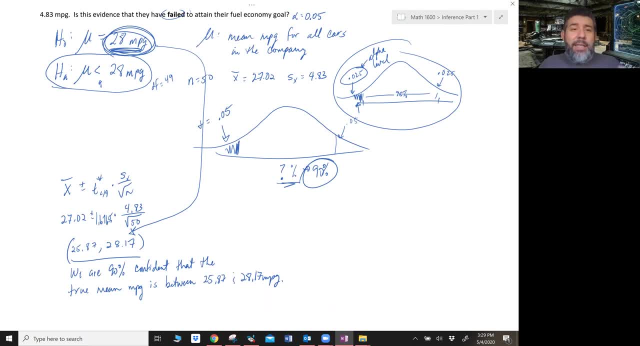 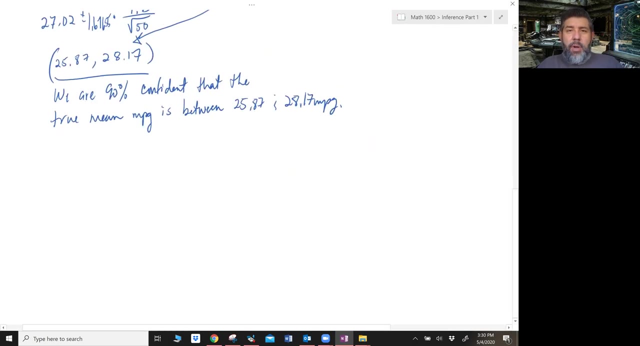 that the um company has less than 28 miles per gallon in their whole fleet of cars. so here's the thing. here's like the whole summary of of this situation. i'm going to zoom in here to kind of summarize this. all right, so if the null hypothesis value 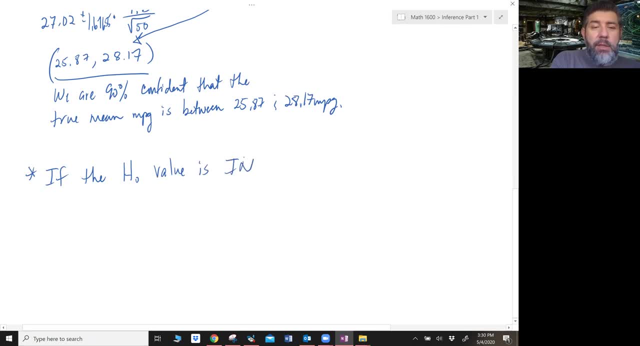 is in the confidence interval, then you're going to fail to reject the null, which means that there's not enough evidence that the alternative is now. that doesn't mean that if the- if the null hypothesis value is not in the interval, do you necessarily always um say, well, we're going to reject the null. so 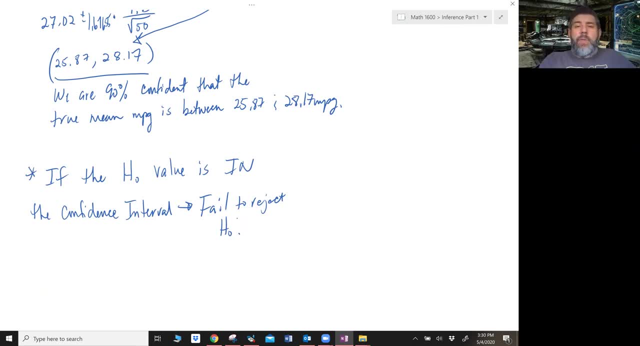 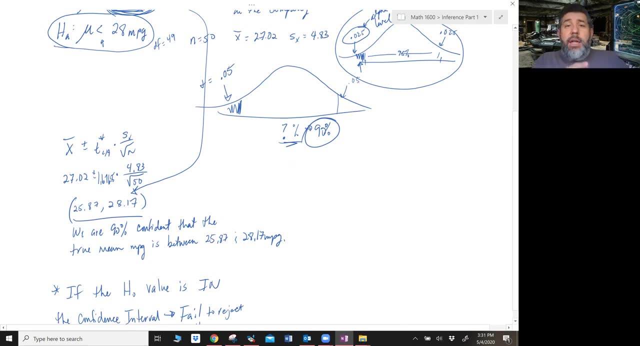 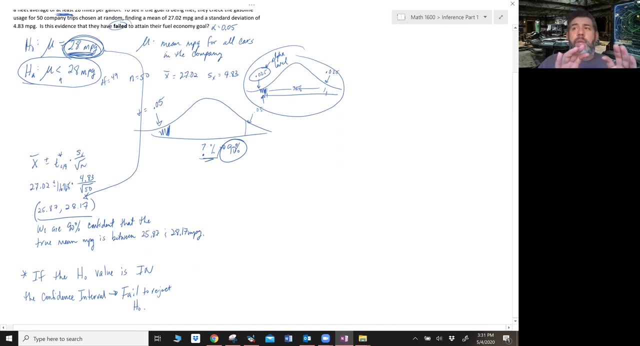 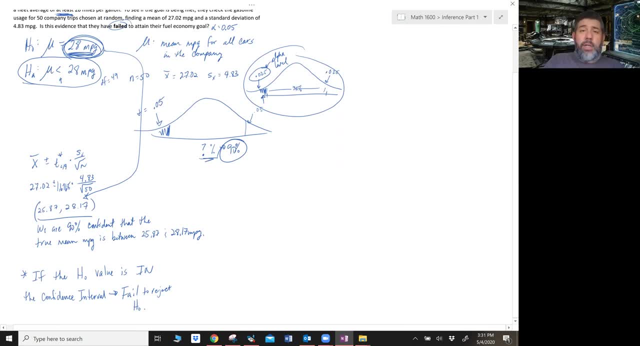 hypothesized value is not in the interval, then we would reject the null because it didn't matter if it's greater than or less than. but we really want to be cognizant of which way the inner inequality is going in the alternative hypothesis, in this particular case, the inequality is less than so we 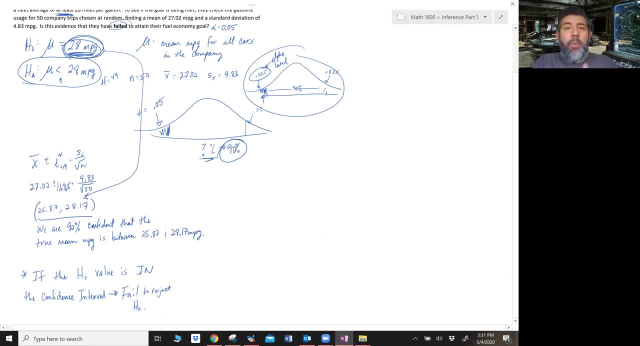 would have wanted to see is, in our confidence interval, both values- the lower end and the higher end- both less than 28? if they had been both higher than 28, then that doesn't really even make sense for what we're doing, for our alternative hypothesis, right? um, in fact, that's even worse. 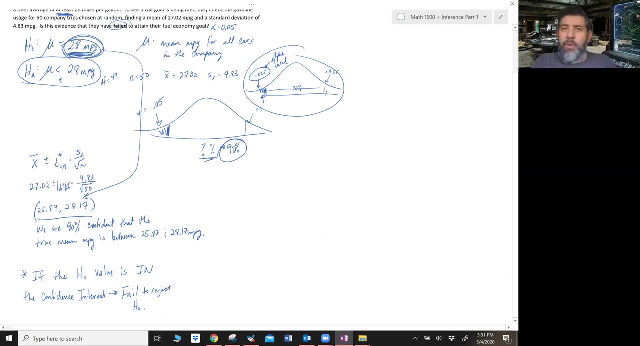 because it's like they really really failed, right. so, uh, most of the time, you're not going to have that case in in a stats class, um, but it is something to be aware of because it might happen in real life. the next thing i want to mention is that this works for. 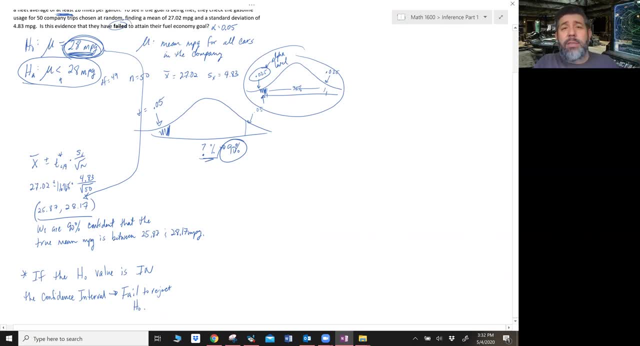 any type of hypothesis test. i used a one sample t interval here, but this would work for a two sample t test. but with a two sample t test you're looking to see if zero is in the interval. so if your interval um changes from negative to positive or positive negative, then you know. 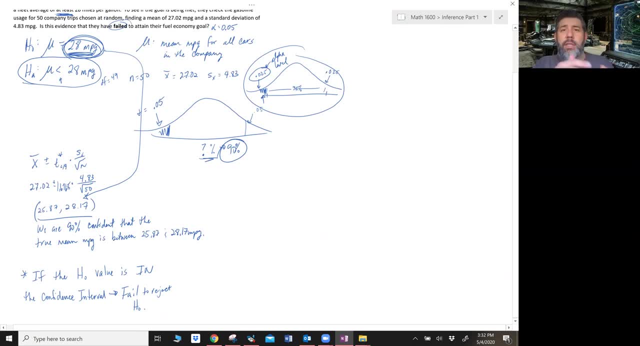 you're either failed to reject- i'm sorry you're, you're um rejecting the null because you're really looking for zero. did i say rejecting the null? if it goes from negative to positive, then you're going to fail to reject the null because zero is within that and that's for a. 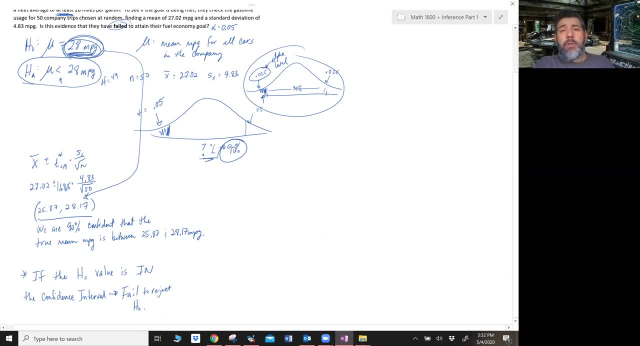 two sample t test for proportions, for inference of proportions. you're doing the same thing for a one um, one prop z test. you're looking to see if the proportion is within your interval. again, it's just, it's all about whether or not the null hypothesized value is in your interval. if it is in your interval, you're going to fail to reject. 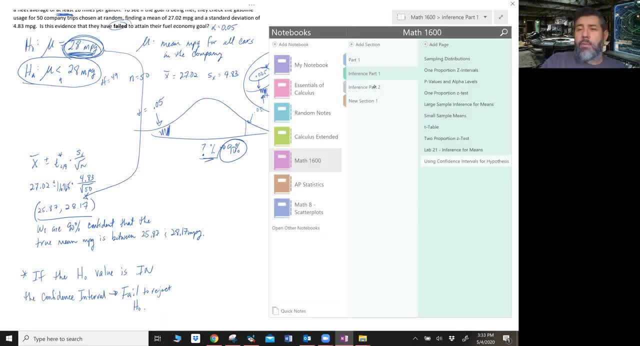 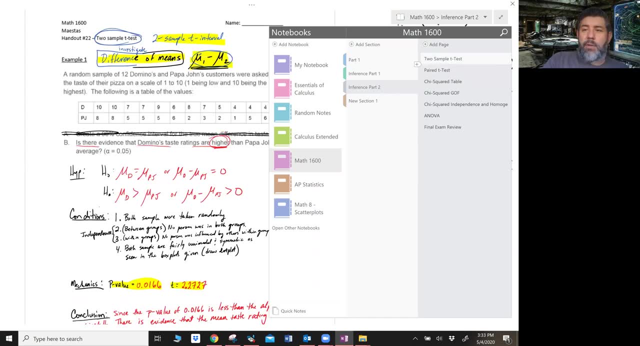 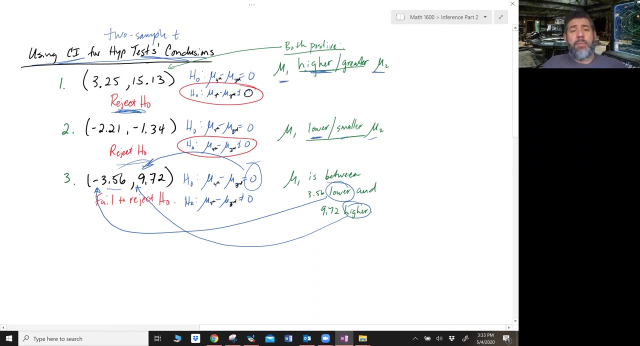 the null and i i think i have somewhere here, somewhere here i i think i did another um. i think i have this written down as well. here we go. here's some examples of that written down. so this is a two sample t test um. so i mean you can take like a little, you know, pause it and take. 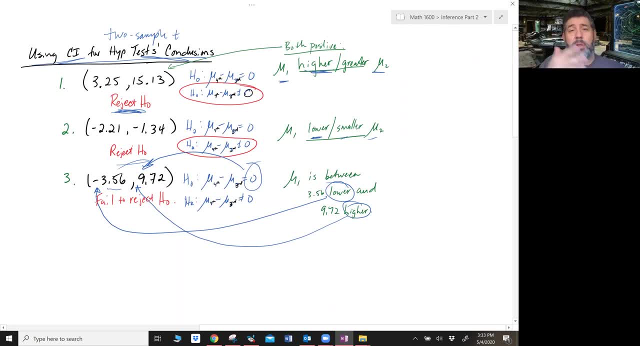 a little snip, if you want. here's some examples of what i mean by: whether you reject or fail to reject the null, and then you're going to fail to reject the null, and then you're going to fail to reject the null based on what that confidence interval interval looks like and what those 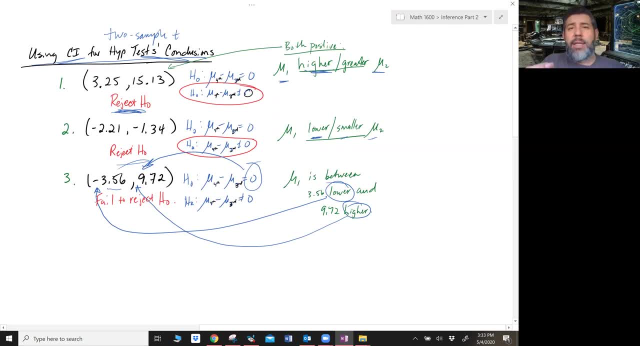 hypotheses might be. so it's really not that difficult, guys, to figure out how to make an inference, um by using your confidence interval. now, this is um. this is particularly important for my students. so for my students, if you, uh, if you do the hypothesis test and you do an entire, 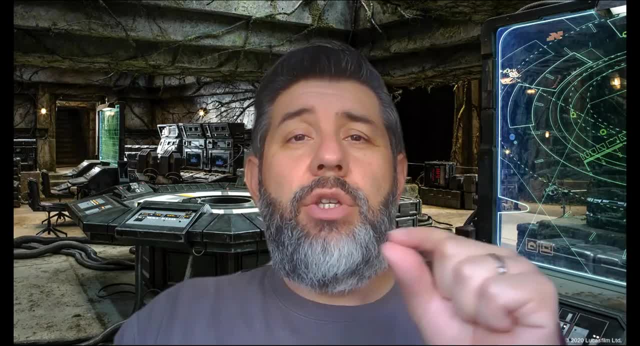 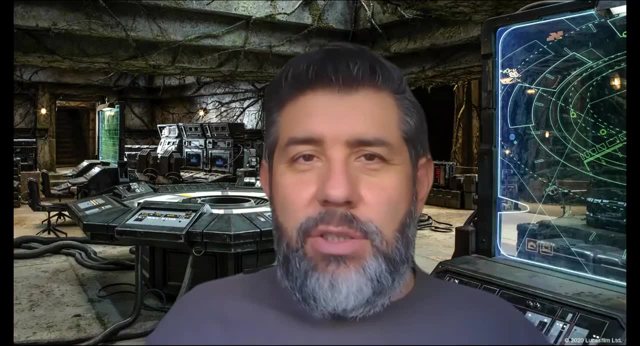 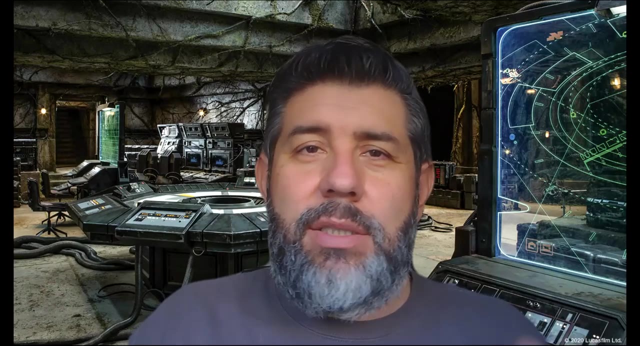 hypothesis test and i ask you specifically, you, you confidence interval to answer the question, then you're not going to get any credit because I didn't ask you to do a hypothesis test. I asked you to use the interval, okay, and that the AP. if you're an AP student watching this, the 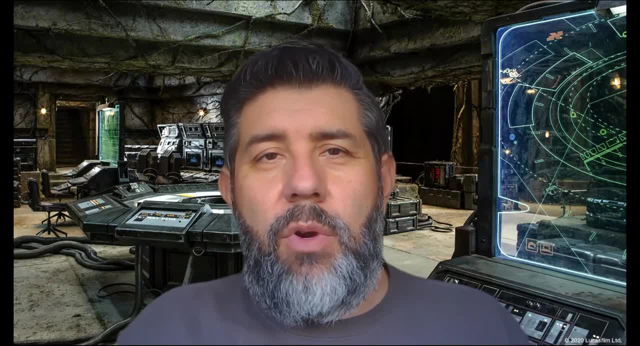 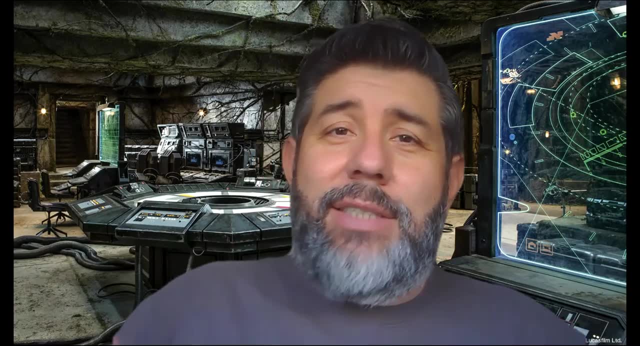 AP statistics exam does that often too, where they ask you about the interval and some people write an entire hypothesis test. you don't get anything, because they're not asking you about the hypothesis test, they're asking you about confidence interval. so do the confidence interval, all right, okay. so that's all. 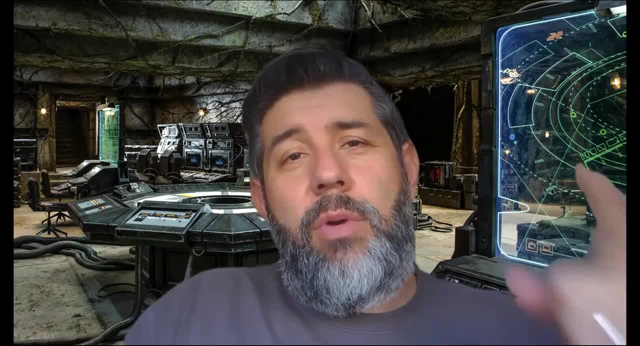 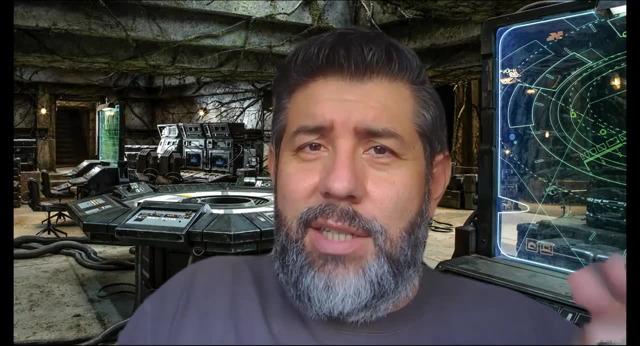 I got for you from the rebel base, all right, and we will hear from you, or see you, or zoom, or whatever else this world has for us. I'll catch you next time. don't forget to subscribe, guys. see you later, bye.